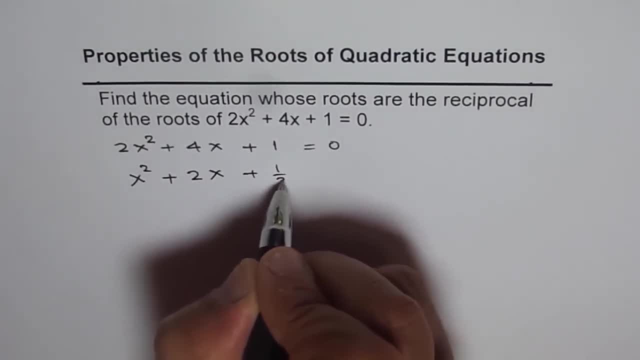 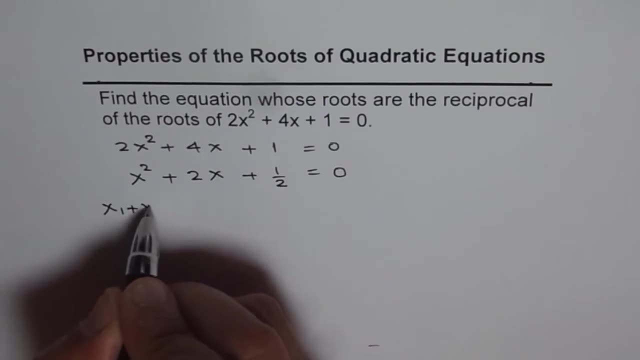 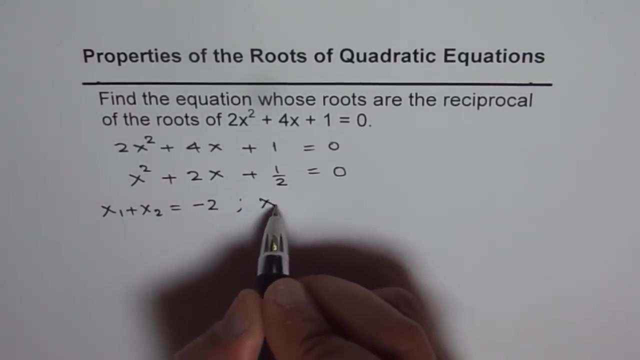 2x plus half equals to 0.. Now the sum of the roots for this equation, that means x1 plus x2, should be equals to negative Of 2, which is minus 2, and the product that is x1 times x2 should be equal to half. Now, 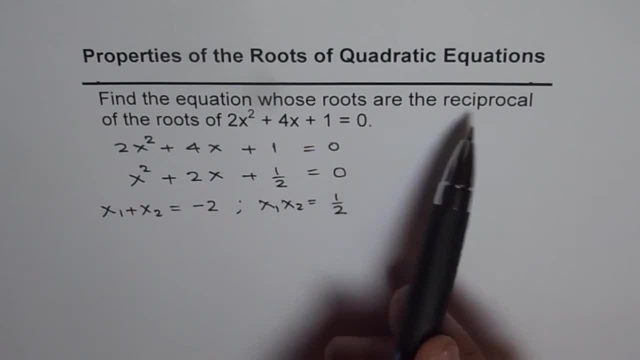 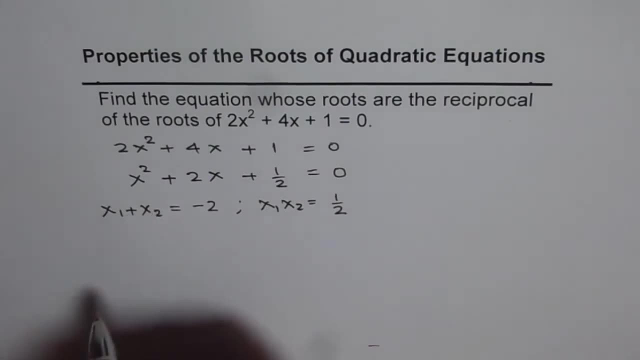 what we need is to find equation whose roots are reciprocal, of these roots. Reciprocal means that the roots will be 1 over x1 and 1 over x2.. So let's find the sum and product of those roots. that means 1 over x1 plus 1 over x2.. 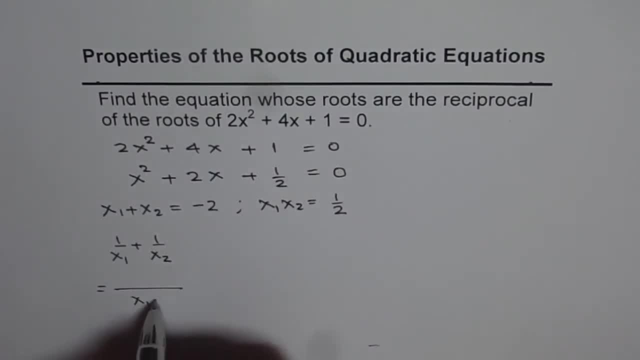 Now that is equal to x1, x2 times x2 plus x1.. Now, since we know, x1 plus x2 is minus 2, so we can solve here. So this is equals to x1 plus x2 is minus 2 over their product. 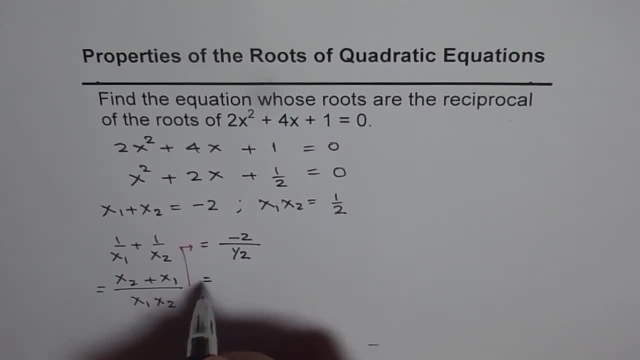 is half, So we write half here, So we get reciprocal sum x1 is actually equals to minus 4.. So that is the first half. Now let us find the product. That means 1 over x1 times 1 over x2.. Now, since x1, x2 is half, 1 over x1, x2 will be. 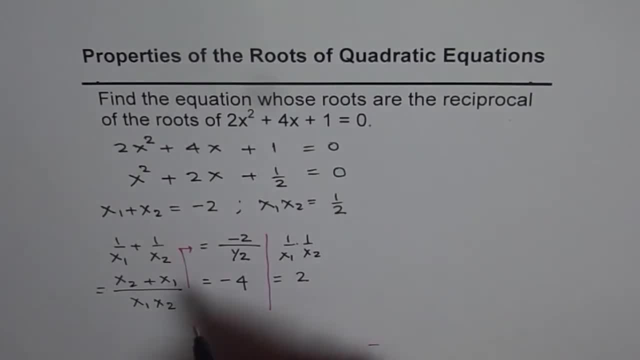 2.. So the product is 2, right. So what we get here is sum as minus 4 plus 1 over x1 plus 4 and product as 2.. And therefore we can write down our equation right. So equation: 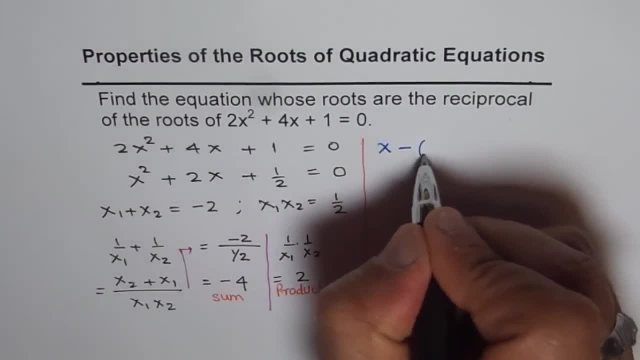 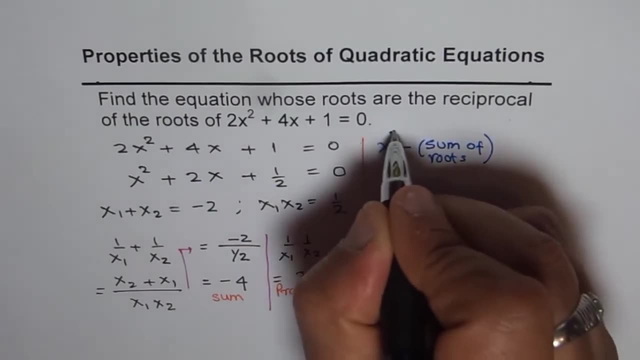 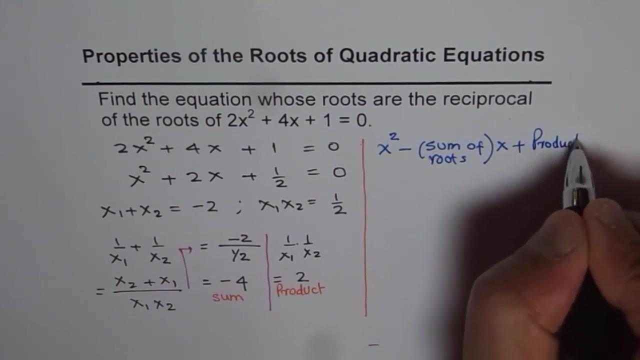 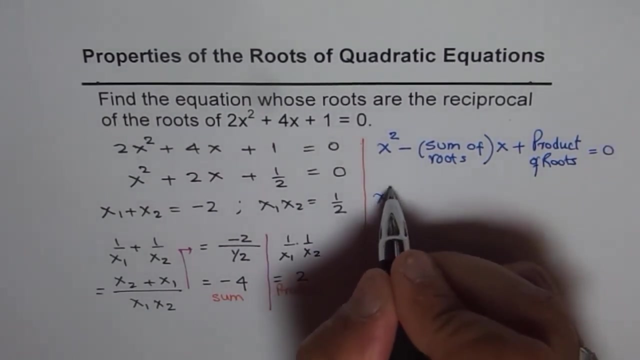 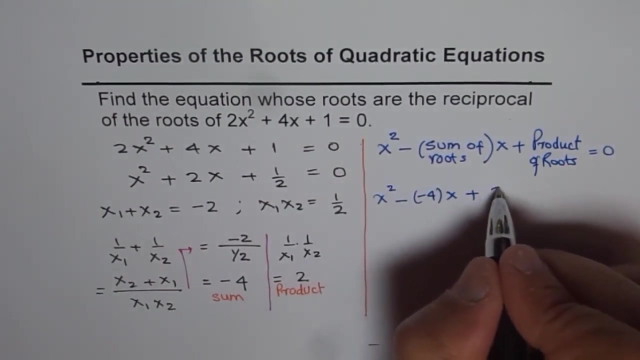 will be given as x minus sum of roots. This is x square minus sum of roots. times x plus product of roots Equals to 0.. So we get x square minus sum is minus 4, minus 4x plus product is 2. Equals.